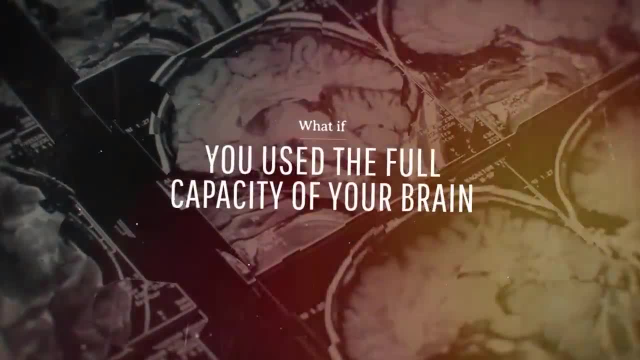 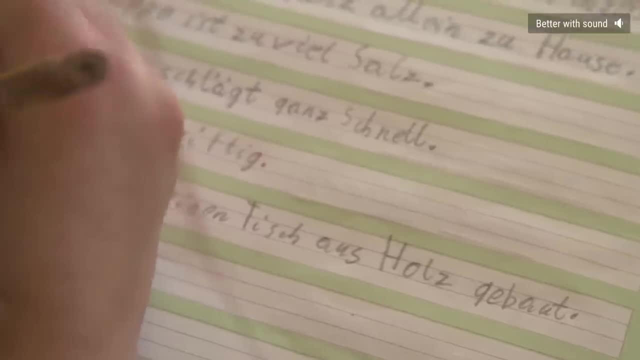 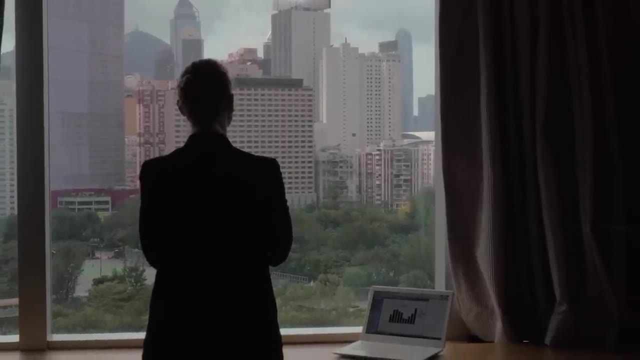 You can do anything: Paint a masterpiece in a minute, Learn every language in an hour, Build a multi-billion dollar company overnight And rule the world by tomorrow. So what's holding you back? Why aren't you doing what you want? 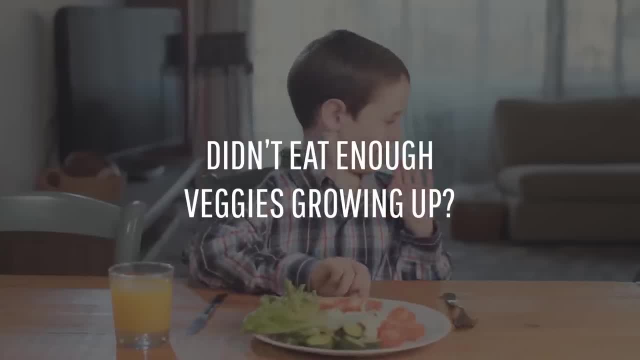 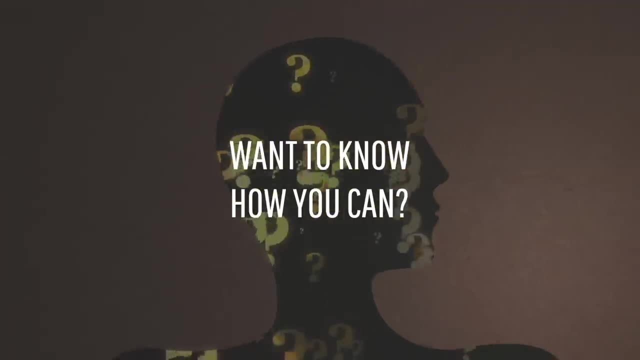 Didn't hear enough Mozart as a baby, Didn't eat enough veggies growing up? Or is it because you're not using your brain at its full potential? Want to know how you can. This is WHAT IF, and here's what your brain would be like. 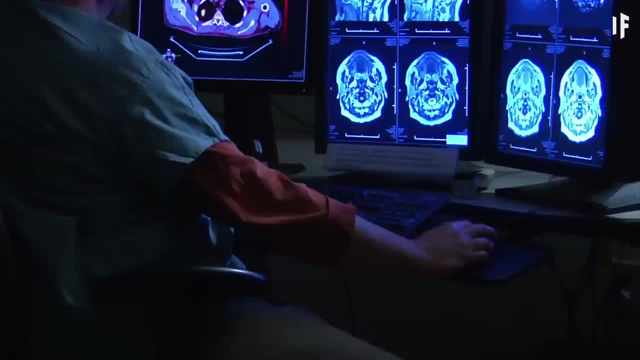 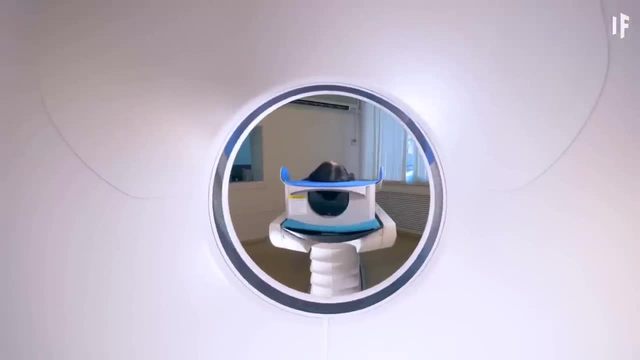 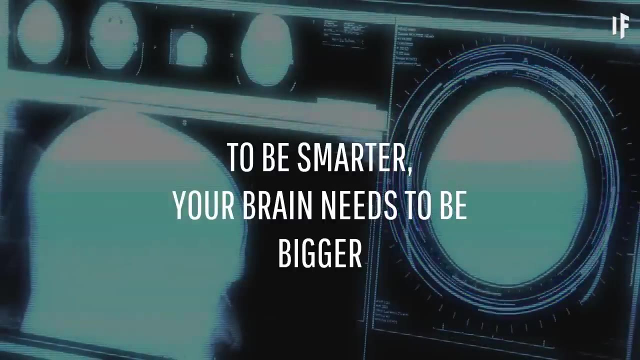 at full capacity. The brain, to say the least, is very complex. We've studied it for centuries and we're still learning more of its secrets today. But be careful: The search for facts can sometimes lead to fiction. To be smarter, your brain needs to be bigger. 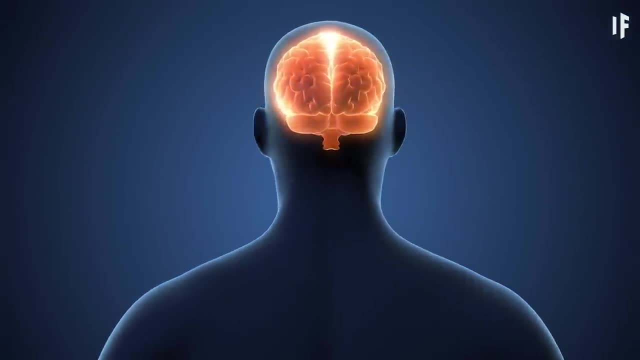 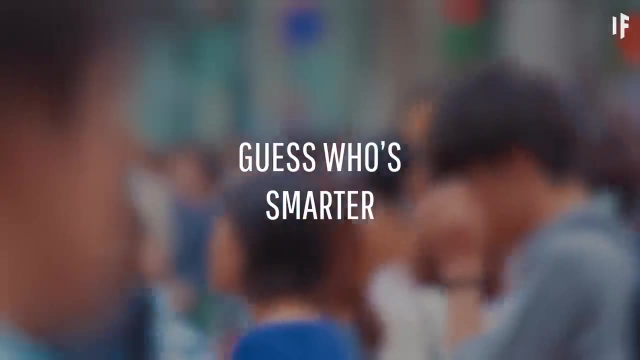 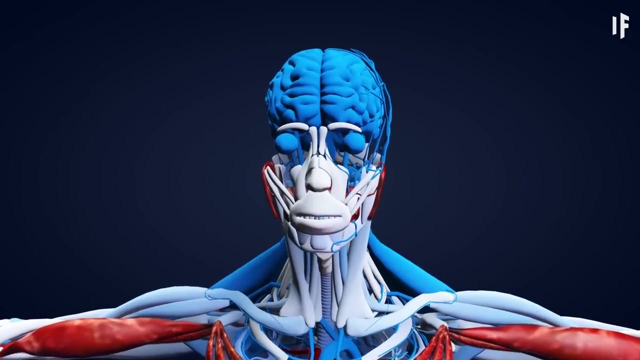 False Brain size relates more to proportion than it does to intelligence. For example, here's your brain next to a whale's. Guess who's smarter. Guess whose body needs more processing power. Your brain is smaller than a whale's because your body is smaller. 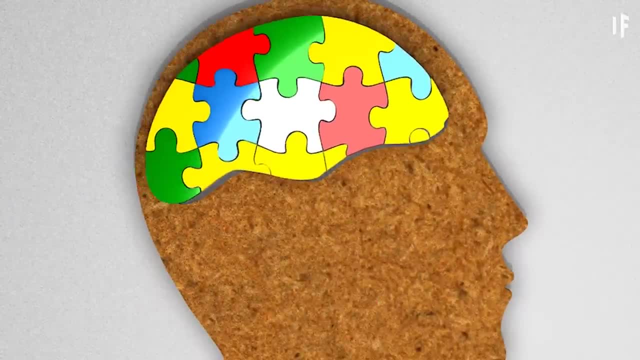 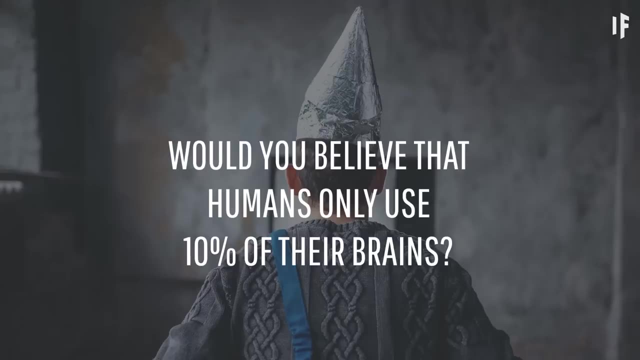 However, your brain is structured in a way that enables you to survive and succeed, But after all, that would you believe that humans only use 10% of their brains? Let's make it 100%. We've seen what really smart people can do. 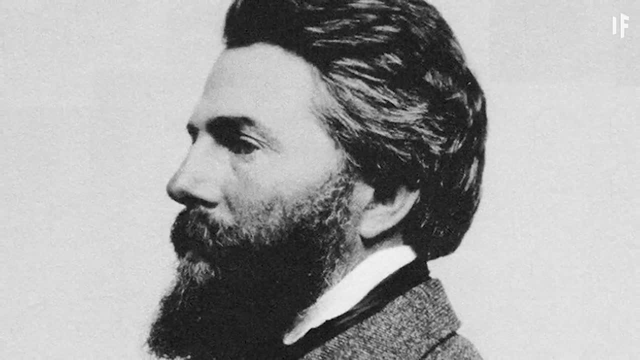 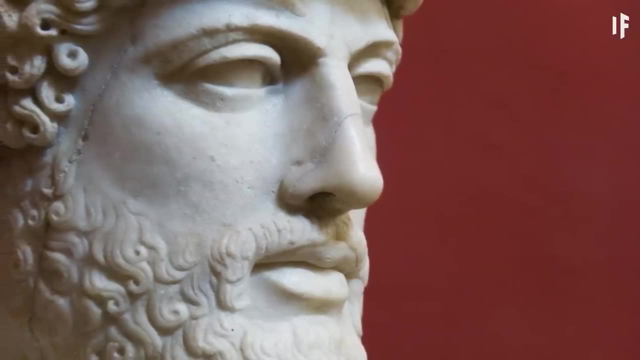 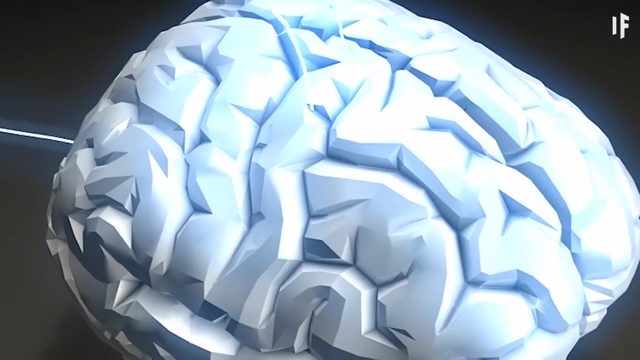 They inspire us through art, music, literature, They change the odds in sports, They come up with tools to make our lives easier And they help organize society as a whole to make us all more powerful, for better or for worse, With access to your brain's full capacity. 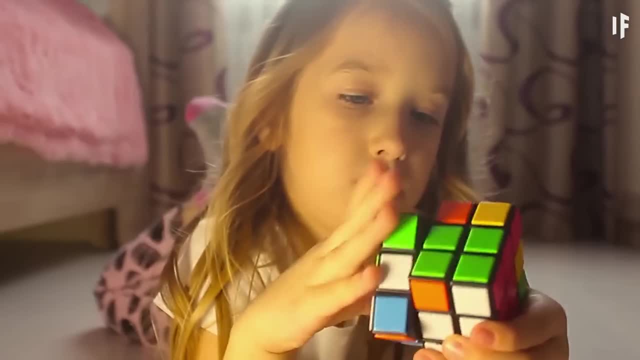 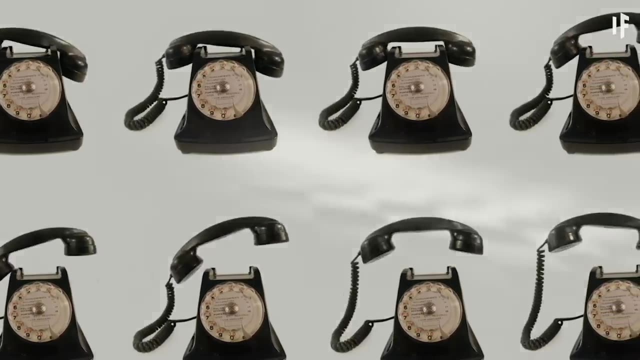 you're limitless. So what do you do? First things first. you finally get to solve the Rubik's cube that's been collecting dust on your shelf. Call up your smartest friend and challenge them to a game of chess. Checkmate in two moves. 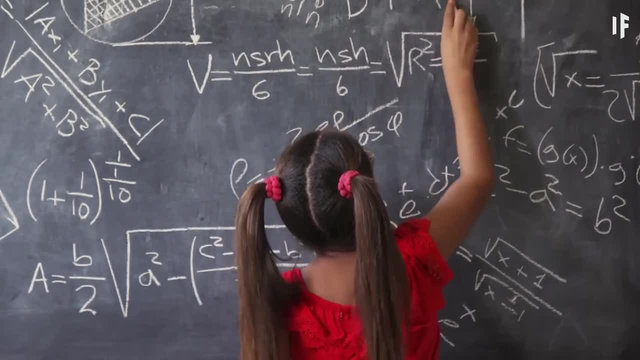 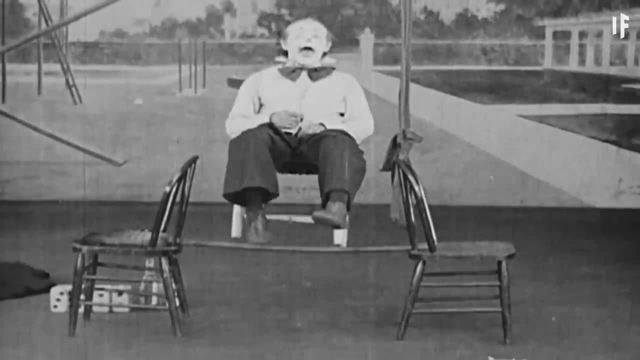 Relish. When you're done being a smarty-pants, you'll be looking for a real challenge, Since being smart means that you won't be as stimulated by the things that keep us simpletons happy. So what's your interest, Art?